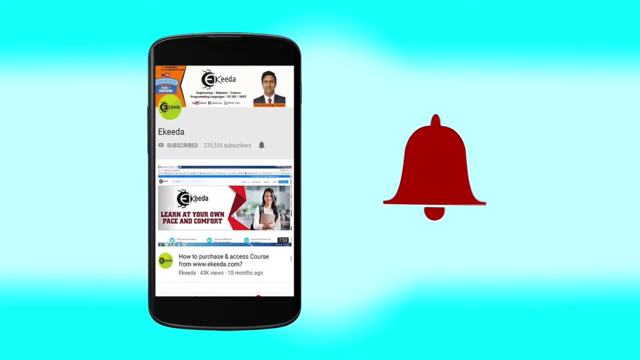 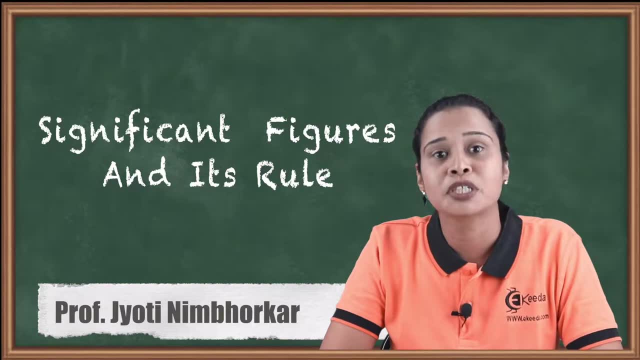 Click the bell icon to get latest videos from eKIDA. Hello friends, today we will see what is significant. figures Now. generally when we do calculation by using calculators, we have a very large number after decimal point and when we go for the further. 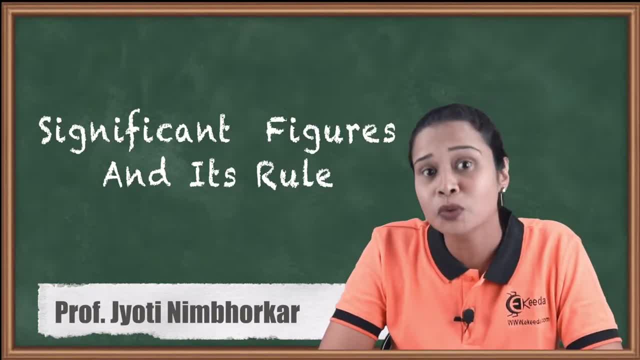 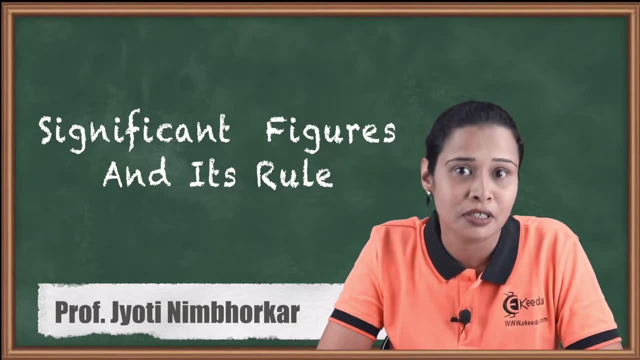 calculation. this becomes very difficult So we have to think where should restrict ourself to find the calculations. So the important part is a significant figure. Significant figure plays very important role in this case. Actually, significant figure is a figure which take important part, or giving meaning to the number, or taking important part for the counting. 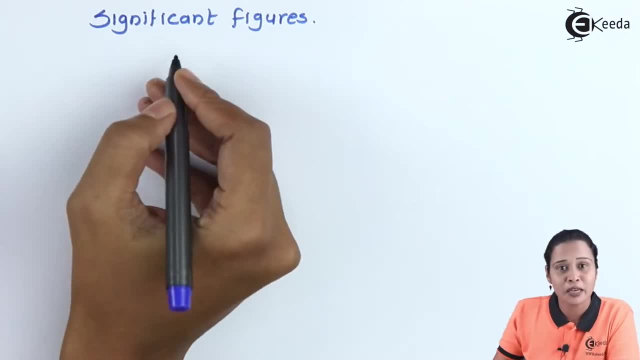 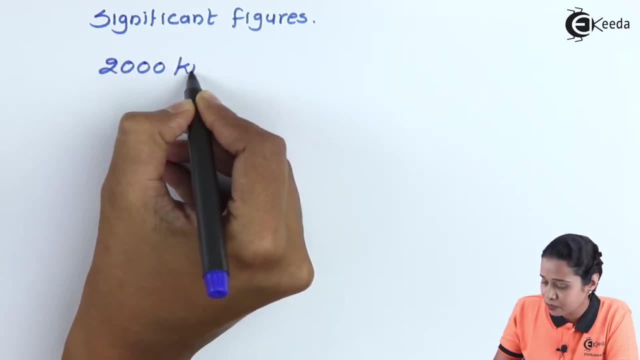 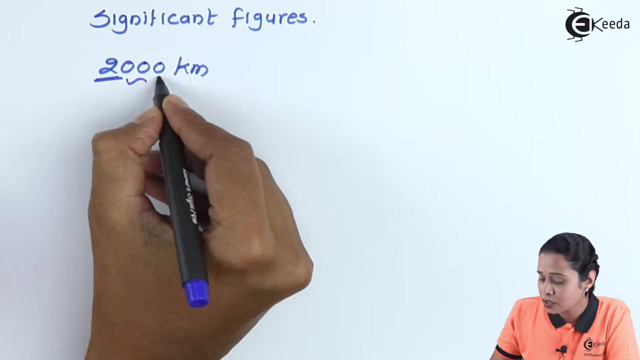 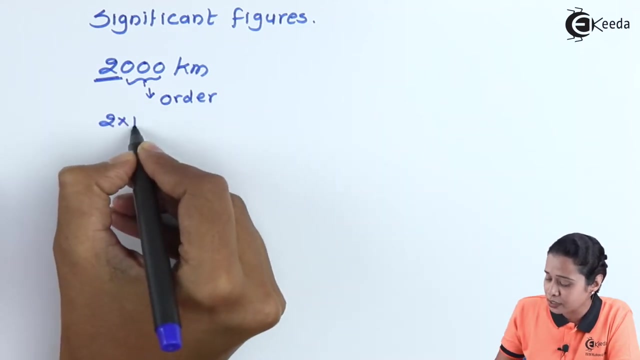 Now let us start with the example. Suppose I am saying the distance of Kerala from Delhi is 2000 kilometers. Now, in this case, 2 is only number which is giving importance. The remaining all, 0, is giving the order. This is the order Means. I can write this: it is 2 into 10, raised to 3, in terms of. 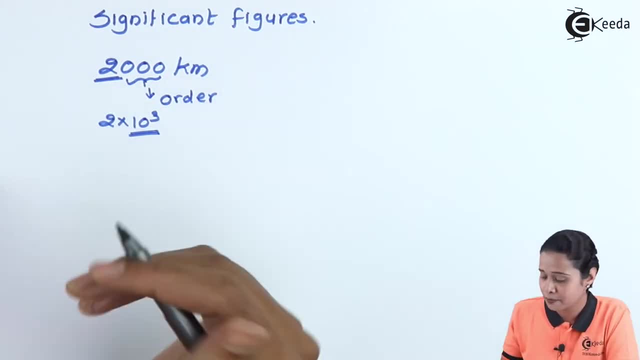 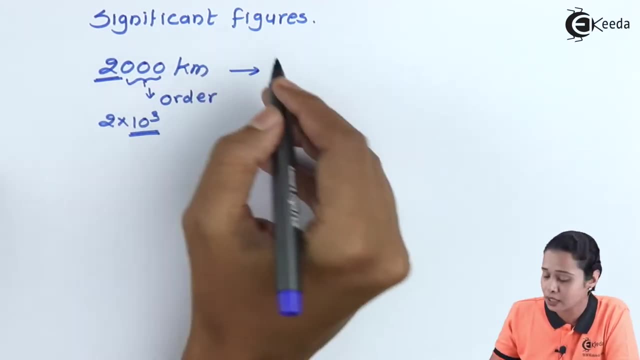 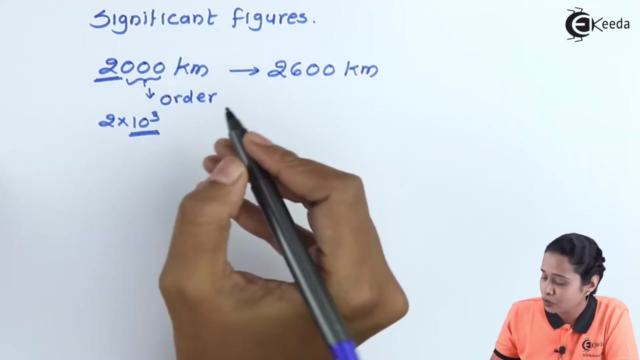 order or it is giving in terms of thousands, But someone is saying this distance more correctly. Suppose another person is saying the distance from Kerala to Delhi, is suppose, almost 2600 kilometers. So in this case we know 2 and 6. both are playing very important role- but other two 0s again. 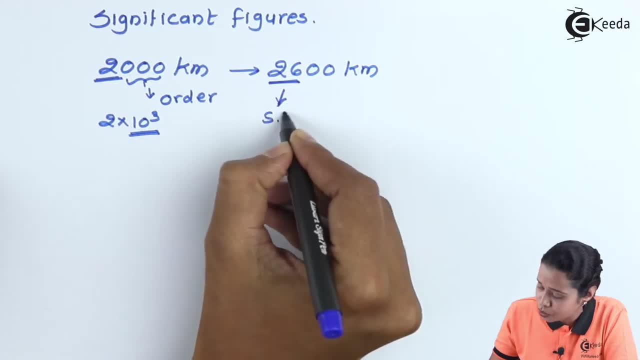 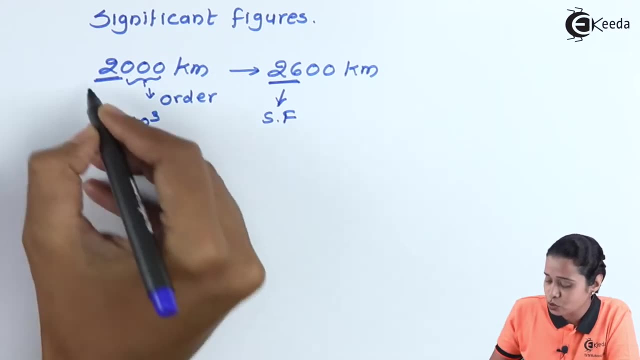 giving the order. So in this case significant figure is 2, while in case of first case significant figure is 1, ie 2. only Now another person comes forward and he is saying the distance from Kerala to Delhi is. 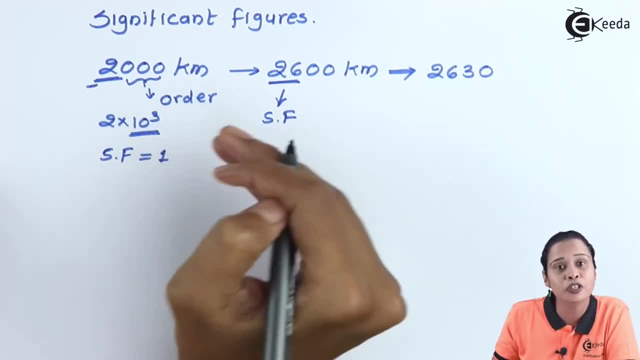 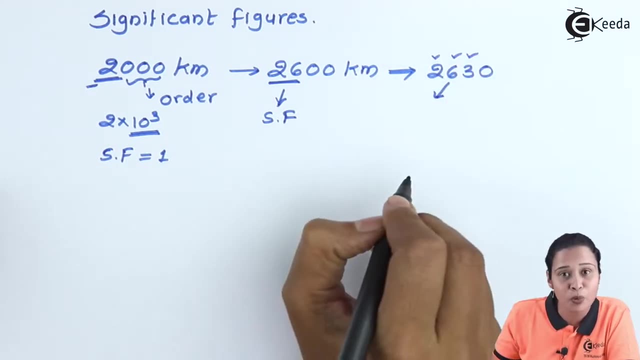 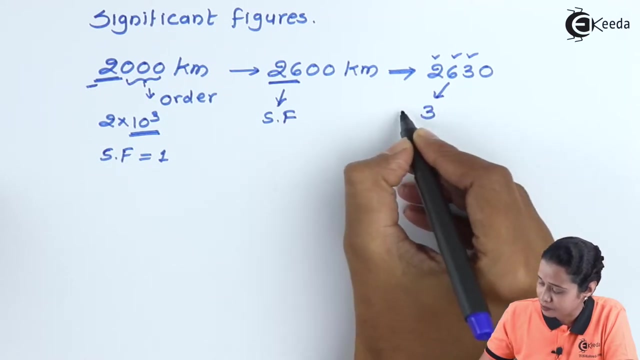 to Delhi is now, in this case, as compared to first, two reading. this reading is more precise means in this case we have a three digits which are playing important role. another one zero, that is giving only the order. So here significant figures are three. Another person giving us a. 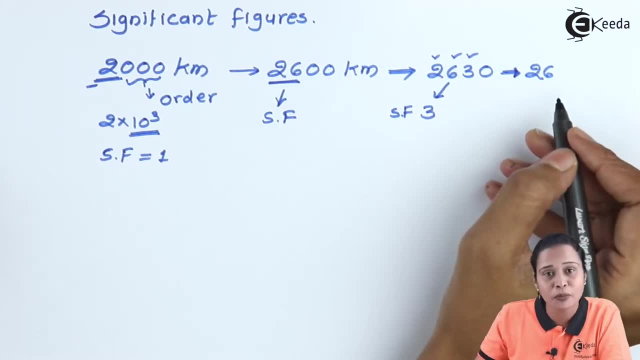 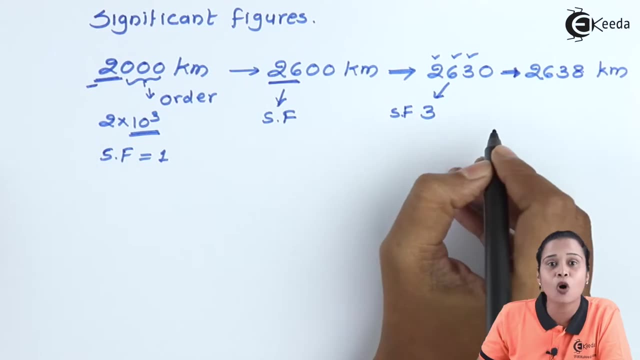 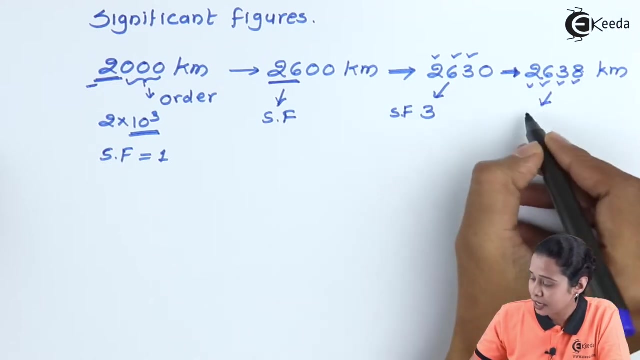 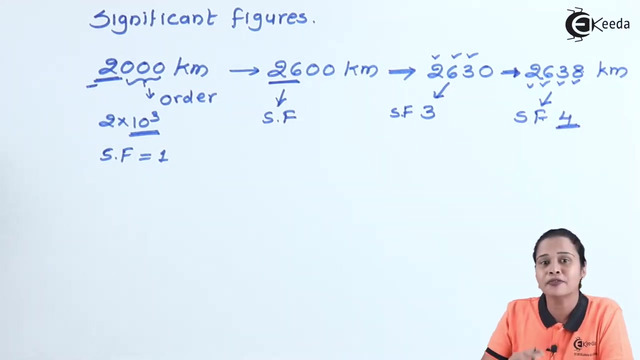 very accurate value and he is saying the distance of Kerala from Delhi is 2638 kilometers. In this case, all four numbers giving a very important values. hence, in this case, significant figure is four means significant figure is a figure which giving meaningful value to the number. Now, 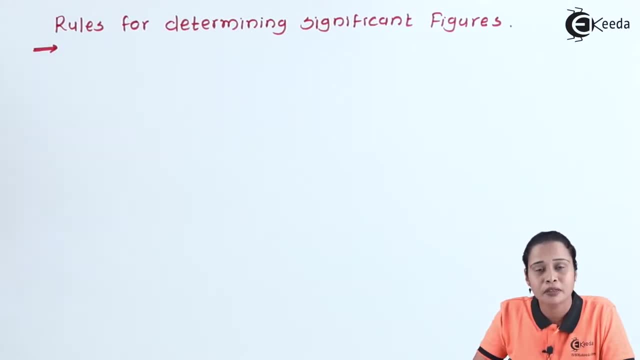 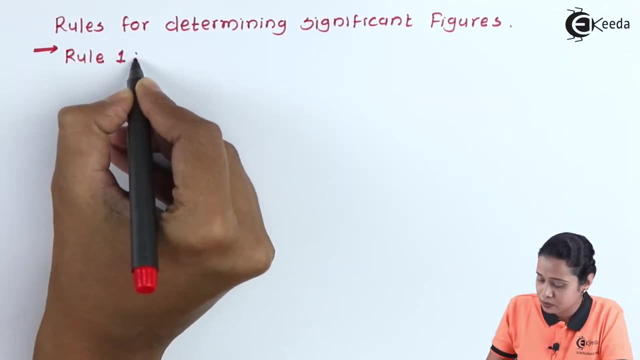 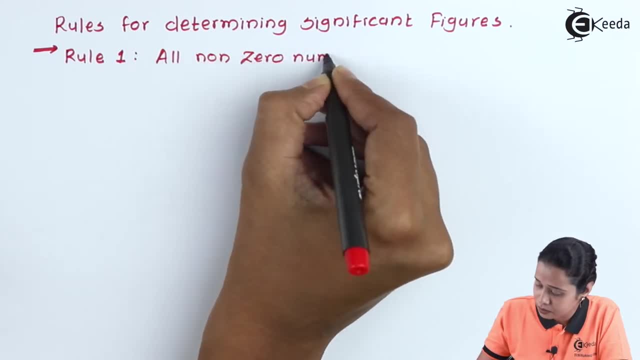 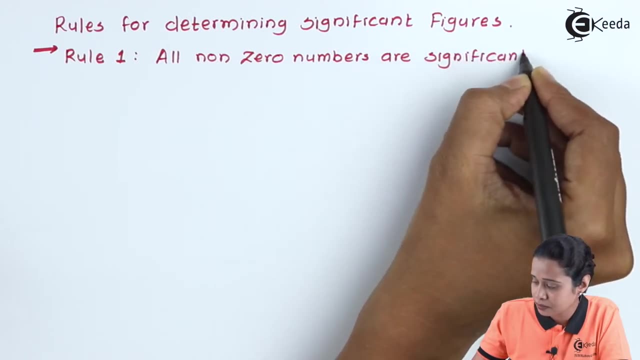 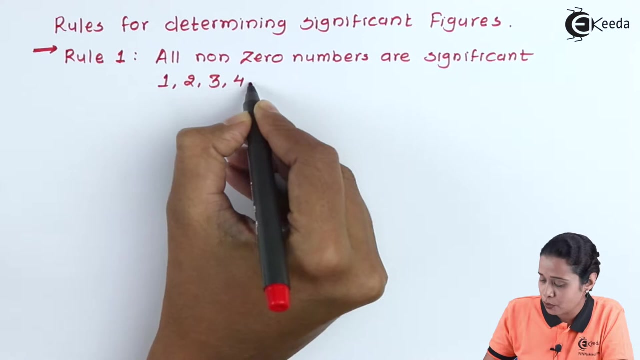 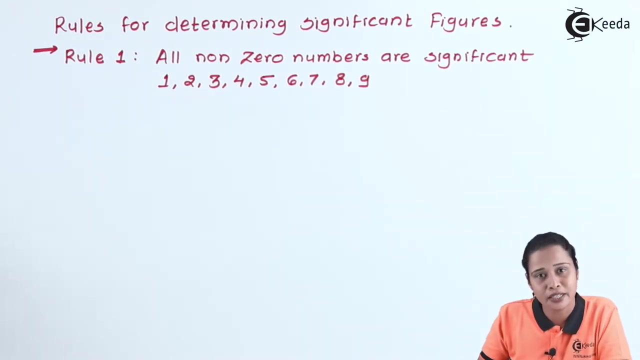 are significant. All non-zero numbers means we can say number one, number two, three, four, five, six, seven, eight and nine. These are the significant figures. Number two: the zeros which are in between the non-zeros number are the significant. 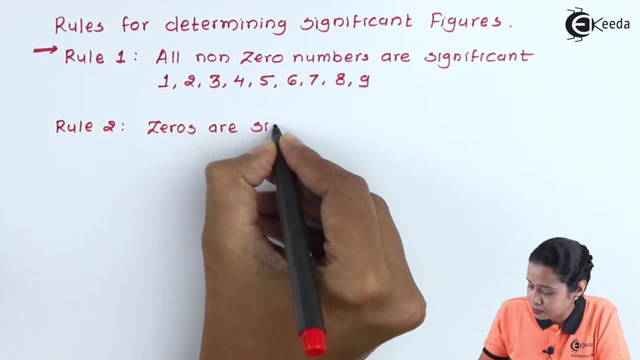 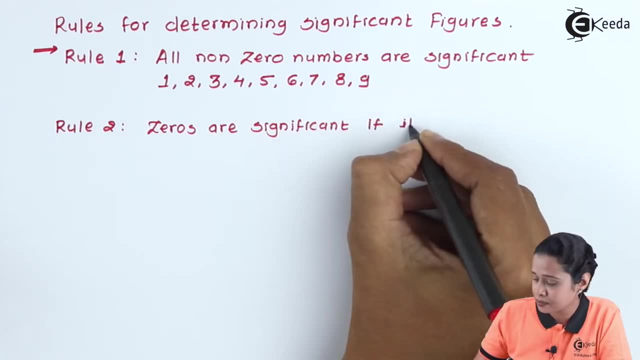 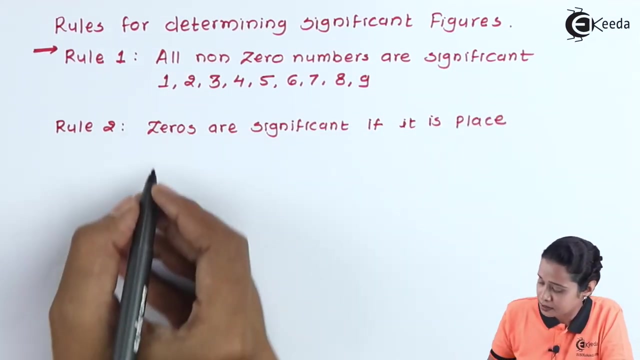 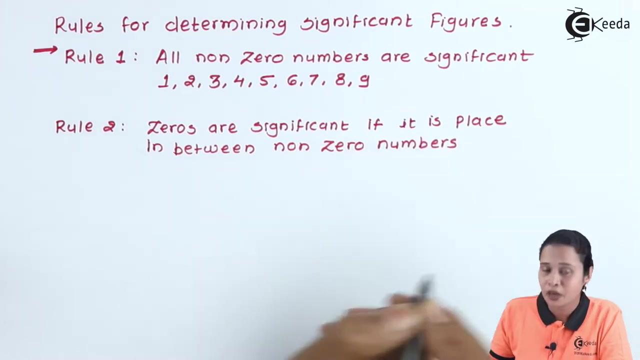 Zeroes are significant if it is place place numbers in between non-zero numbers. For example, if we are saying the number 1,, 9,, 0, 2.. In this case, this 0 is placed in between these two non-zero number, Hence the significant figure. 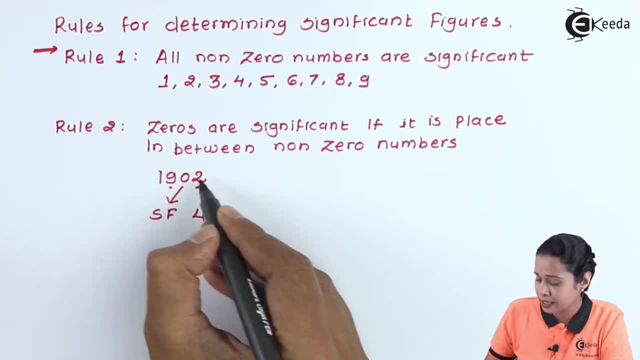 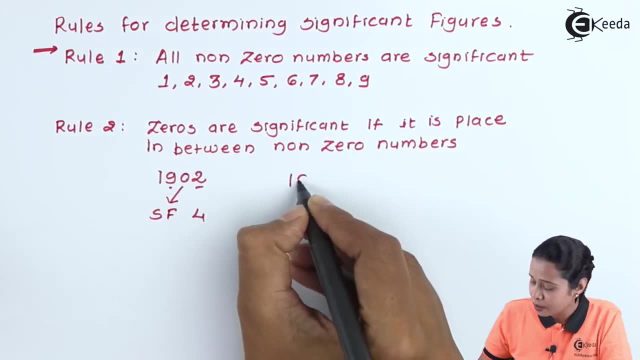 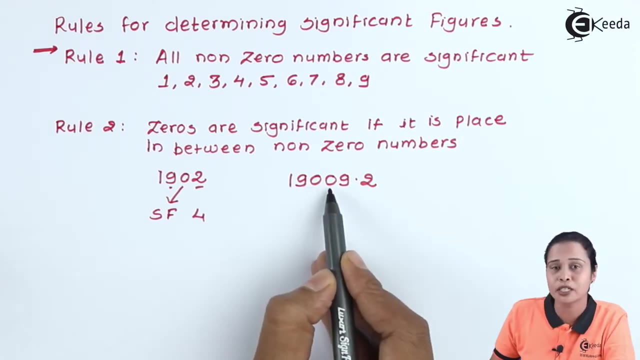 in this number is 4.. First, second, third and fourth means 0 is also a significant figure. We can take another example. For example, we have 19009.2.. In this case, again, both the 0s are. 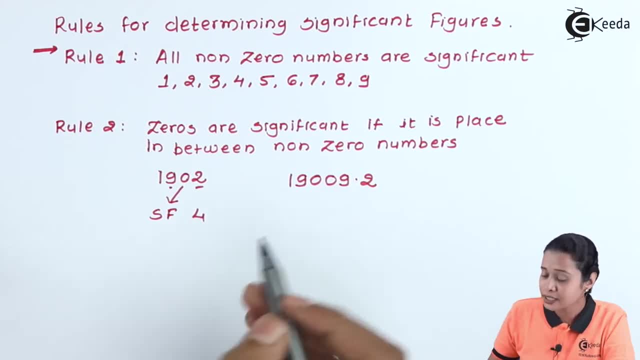 placed in between the two non-zero number. Hence, in this case, significant figures are 1,, 2,, 3,, 4,, 5 and 6.. There are 6 significant figures, So 0 can be considered as significant if it is placed in between the non-zero numbers. 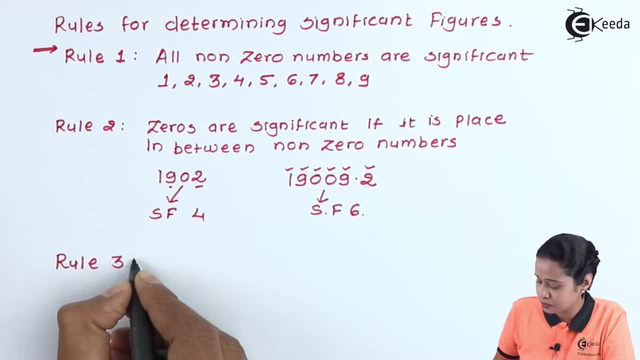 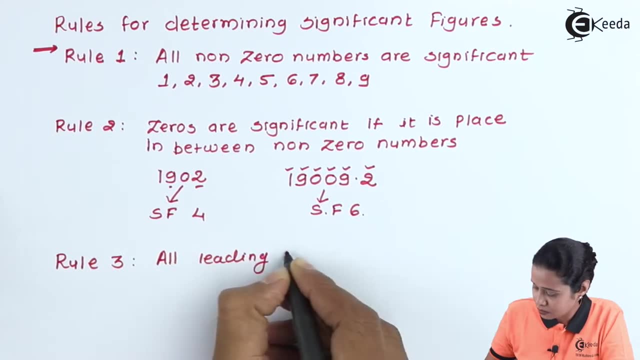 Let us start with rule number 3.. All leading 0s are insignificant. We can take some example of this. For example, we will take 0.2.. Now here we have a 0. The position of 0 is a leading. 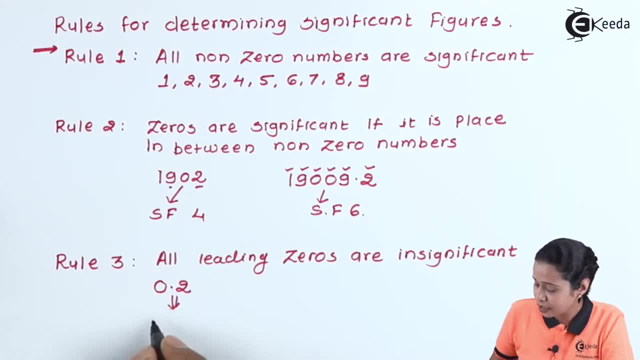 position. But I can express this term in this way: 2 into 10, raise to minus 1 means it is giving, that 0 is giving the order. So in this case significant figure is only 1.. That is 2.. Let us take another example. Suppose we have another number that is 0.05.. So we: 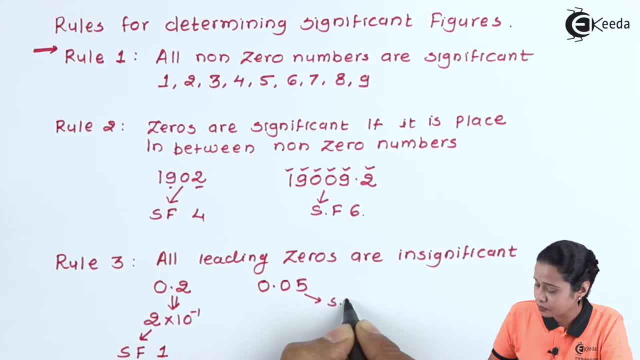 can take 0.2.. Again, significant figure is 1.. That is 5 here. Why? Because again we can convert this number in this way: 5 into 10, raise to minus 2. Means, again these 0s are giving the order. 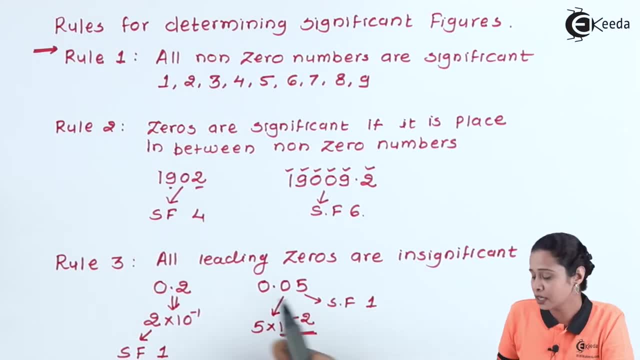 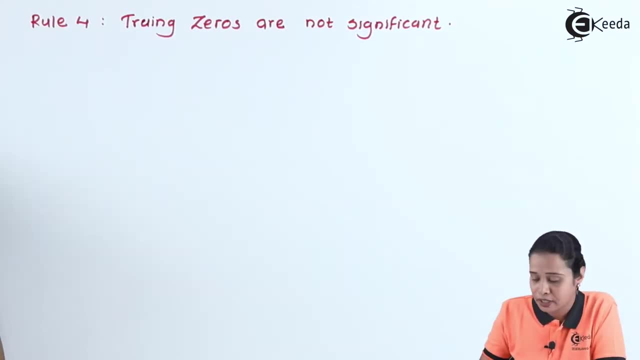 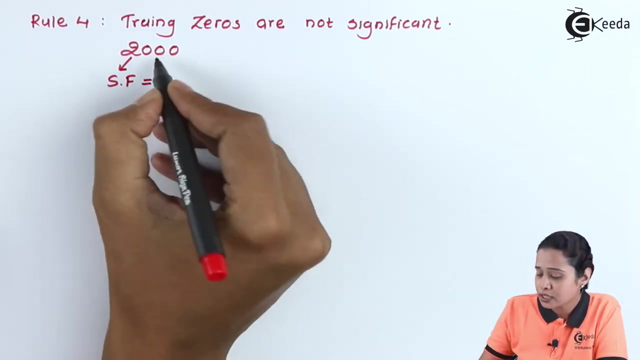 Means here. in such a example we cannot consider that 0s are significant. Let us start with rule number 4. Trained 0s are not significant. Let us take some example of it. Here we have a number 2000.. Then in this case significant figure is only 1. That is 2. Because 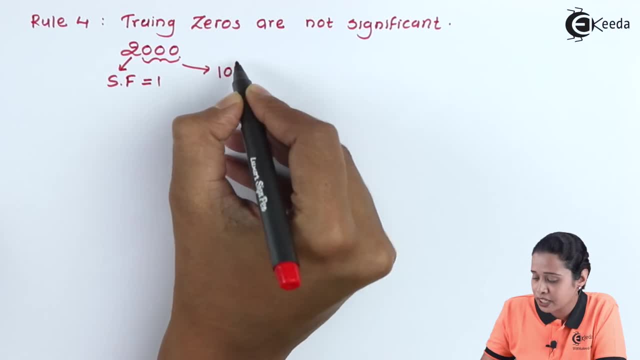 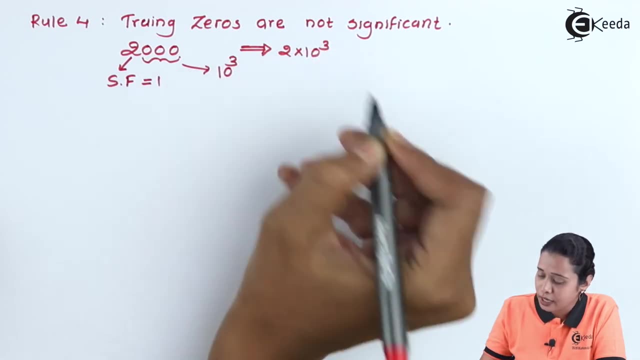 this remaining 0s giving us a order. We can say: this is 10 raise to 3. Means. we can write this number in this way: 2 into 10 raise to 3. Hence, significant number is only 1. Means. 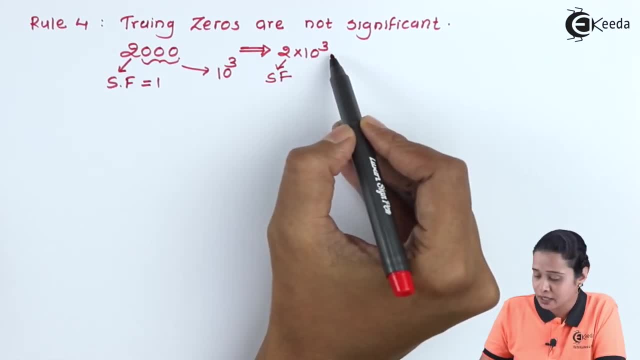 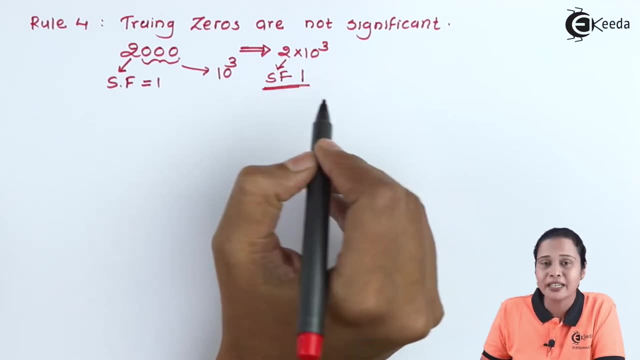 we can convert this number in this way: 2 into 10 raise to 3. Hence, significant number is very similar to that. So this number does notdled the order. That is why in rule number 3.. Now let us know right now. 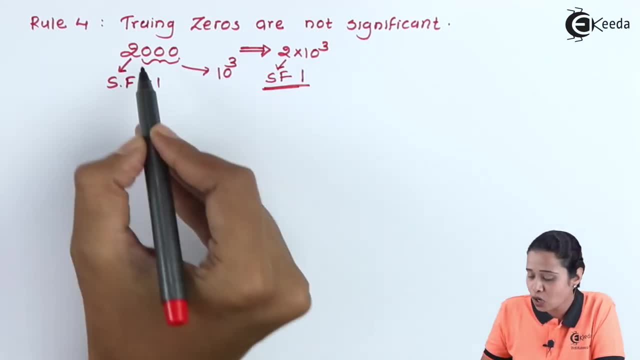 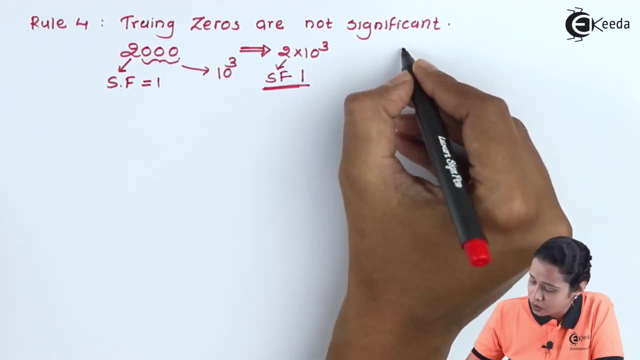 First, what are these 10 raise to 3?? They mean the number of человек inside a set of tables, or how we can understand their order. 10 raise to 3 is given by the 0sする to 1.. So~ 1 raise to 3 is relatively simple. 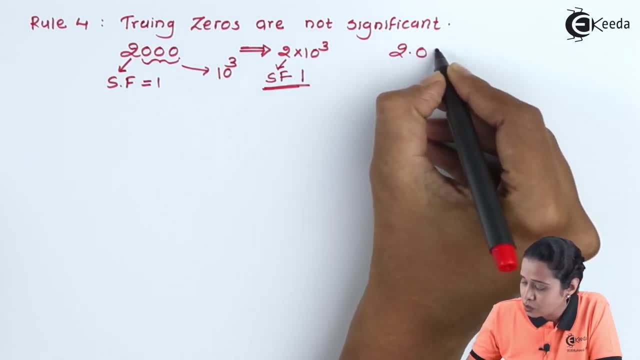 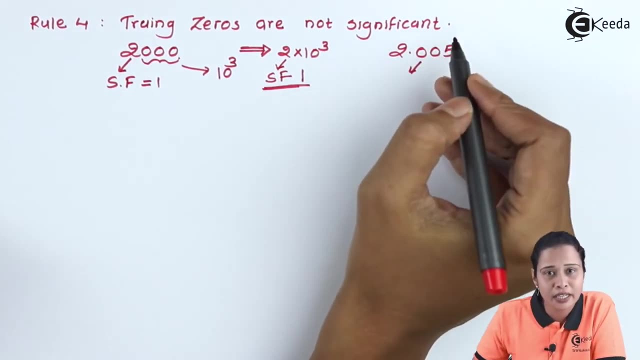 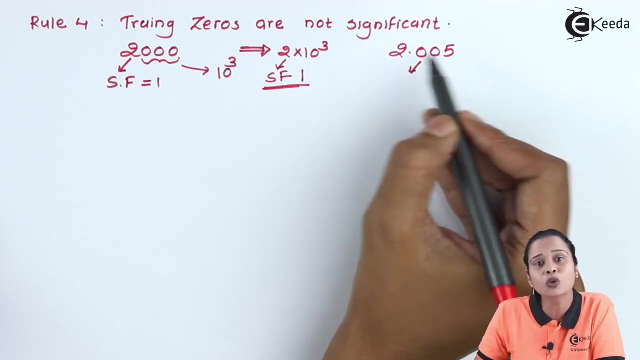 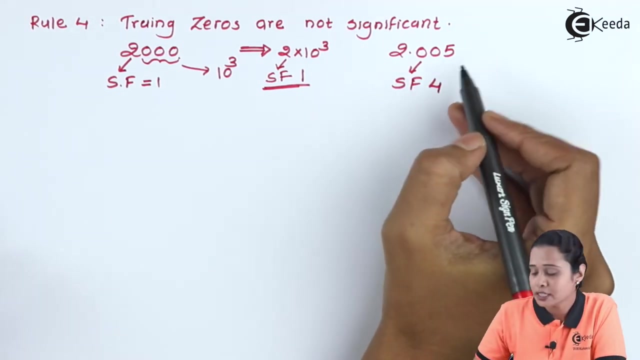 That is what we have calculated, Otherwise nothing. many who have come to this Suppose we are taking another example, that is 2.005.. In this case we know the zeros are in between the two non-zero number. That is why here we will say: significant figures are 4, because these two zeros are also treated. 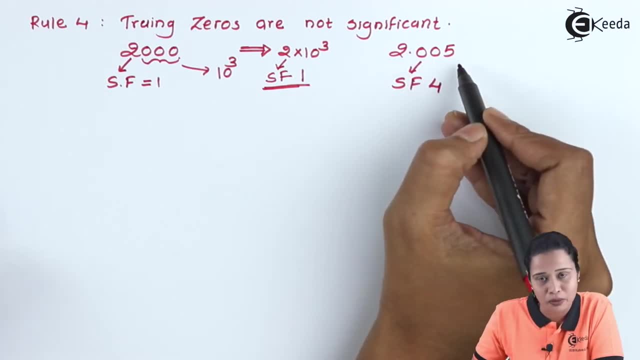 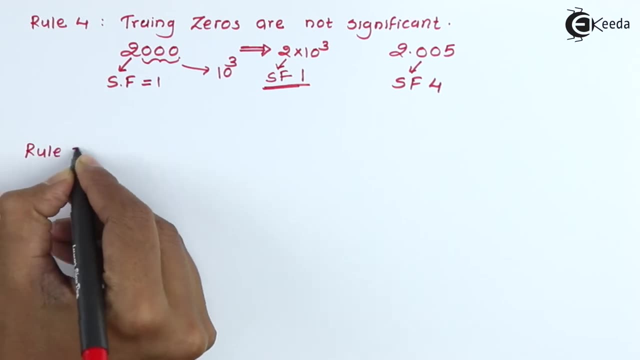 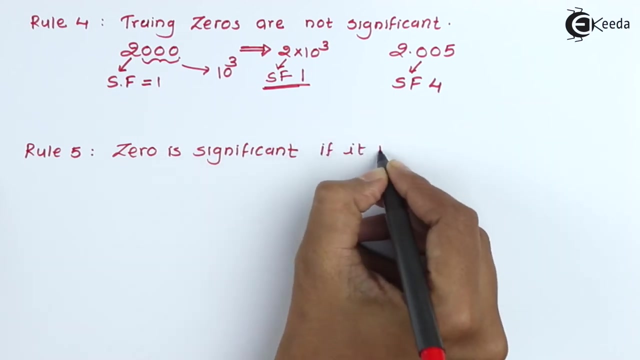 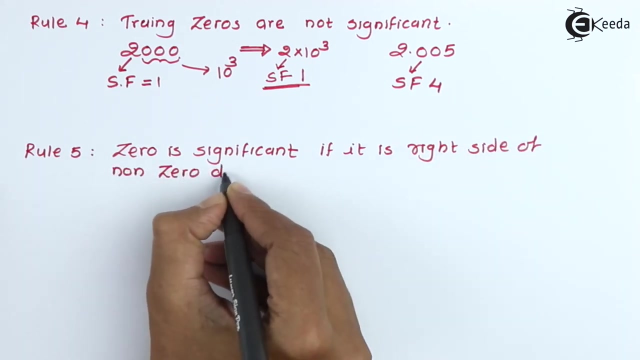 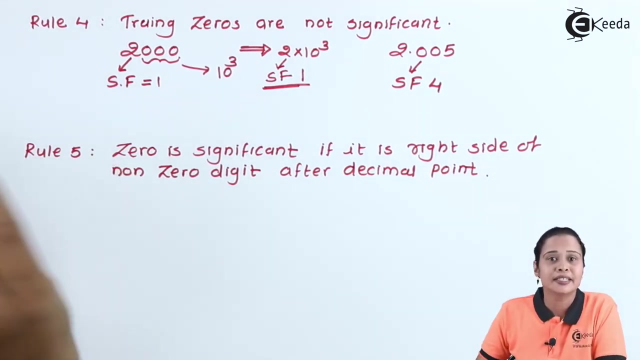 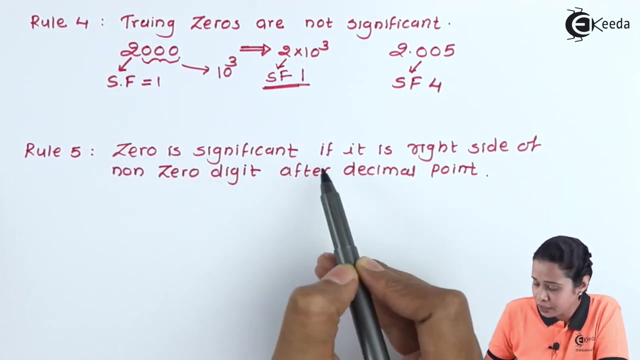 as a significant because it is placed in between the non-zero number. Let us see what is rule number 5 for significant figure. Now, rule number 5 is 0 is significant if it is right side of the non-zero digit after the decimal. 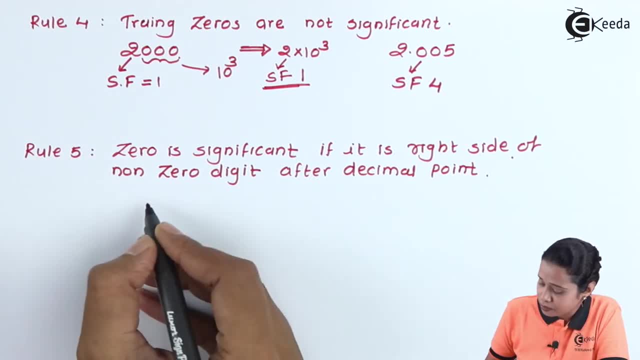 Means. we can take one example. Suppose the example is 0.2300.. Now, as per this rule, these two zeros are after the non-zero digit of the decimal point Means. here we can write: this significant figure is 4.. 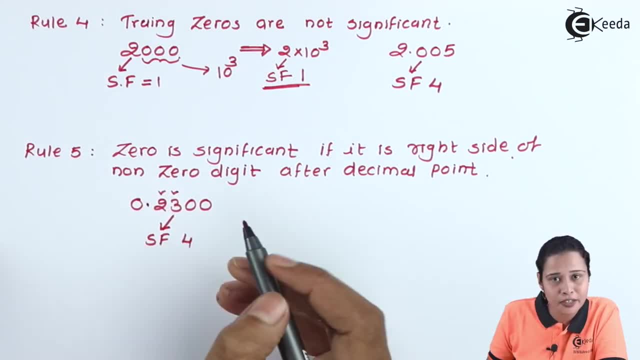 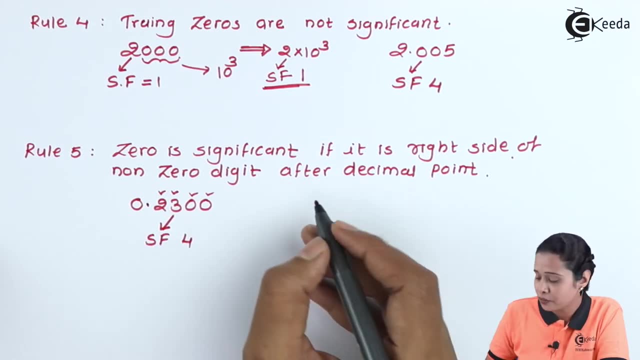 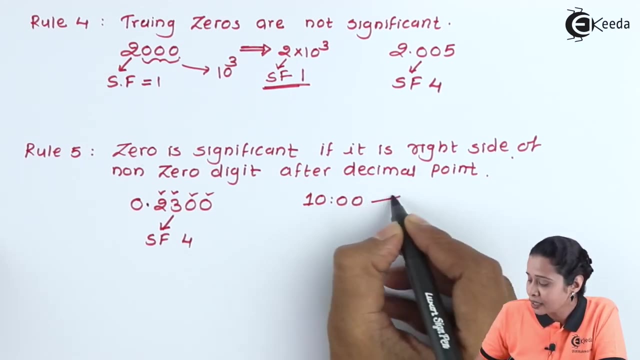 Means all these two digits are significant, as well as two zeros are odd. So these two zeros are also significant. because, suppose someone ask you time, we can say time is 10.. We will write down 10.00.. It means time is not 9.55 or it is not 10.05.. 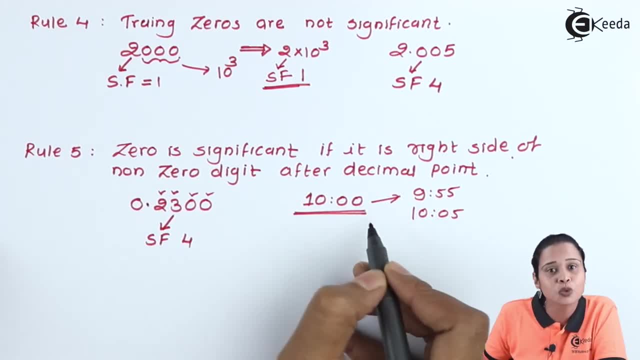 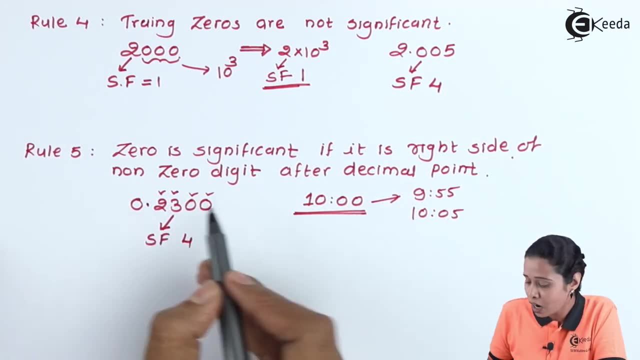 Time is exactly 10.. That is why these two zeros are also playing very important role in the number. That is why, when, whenever there is a zero after non-zero, digit After decimal point will be considered as the significant number. We can take another example. suppose we have 0.00500. in this case, what is the significant? 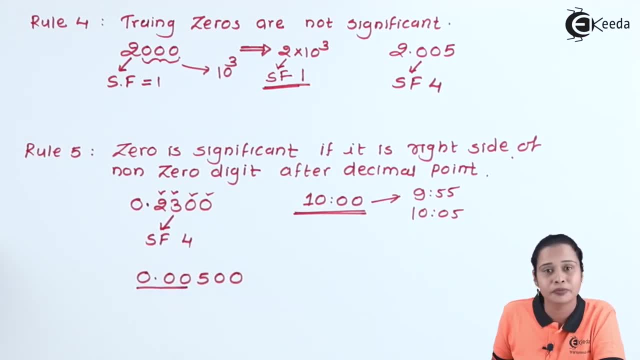 figure. Now, these two zeros are leading zeros. That is why we cannot consider that zeros as a significant number. but these two zeros we have to consider as a significant number because it is giving us a proper number. Hence, in this case, significant figure is 3..